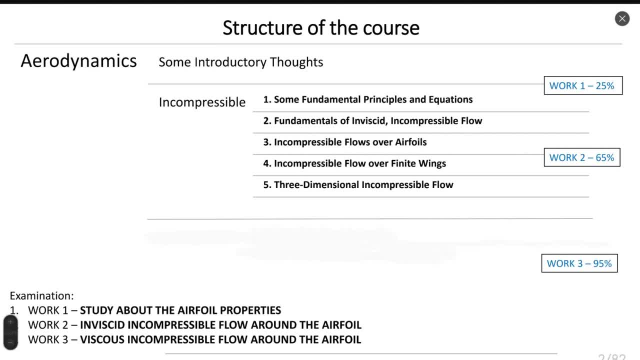 Incompressible flows over airfoil where we discuss theory of thin airfoils and cambered airfoils, trying to apply Laplace's equation for real airfoil structures. Then we talk about flow over finite wings, where will be introduced a question of three-dimensional flow around the wing with side effects and at the end of the course we will talk about three-dimensional incompressible flow model and introduction to numerical techniques 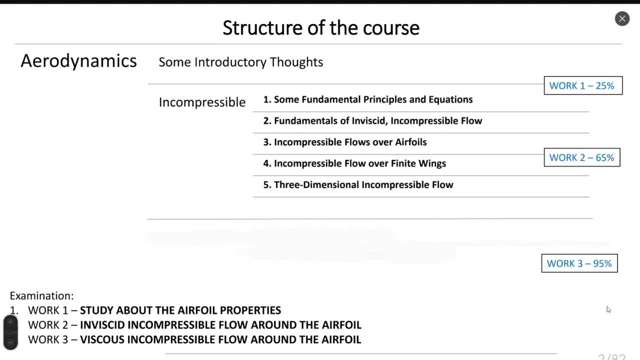 based on solution of Laplace's equation. The course of aerodynamics has 60 hours of lectures and 15 hours of practical classes. 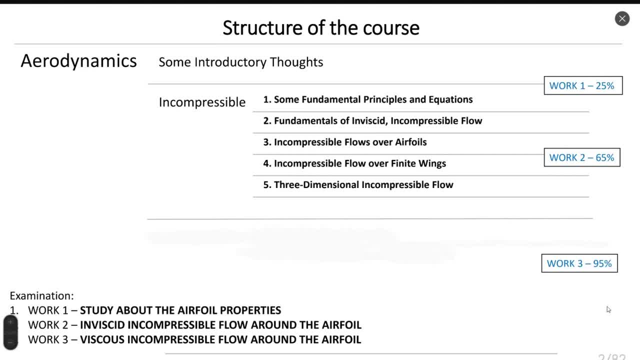 Practical classes are a solution of numerical problems in Ansys Fluent which I recorded separately and you can find them on my channel as well. During study of aerodynamics you will need to make three works. Work one is about study of the airfoil properties. 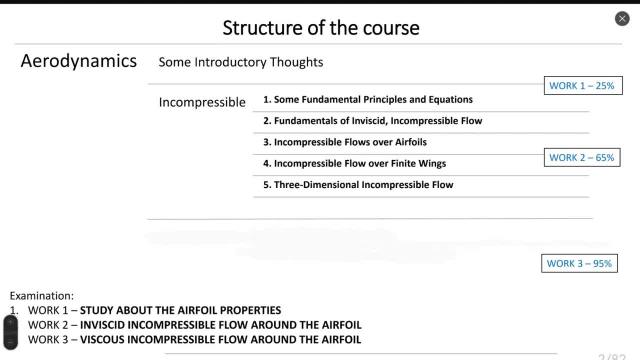 It must be delivered at one quarter of the course. Work two is devoted to simulation of inviscid 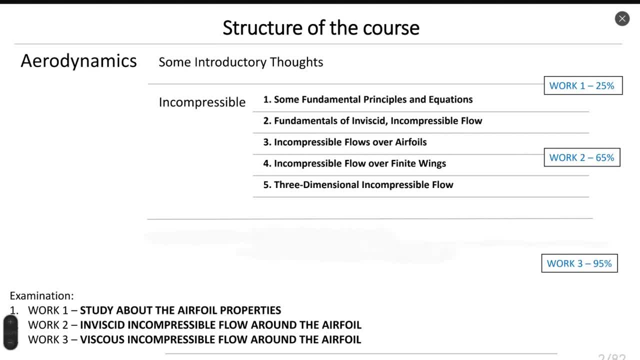 flow around the airfoil. It must be delivered at 65 percent of the course. And work three is about numerical simulation of viscous incompressible flow around the airfoil. It must be delivered 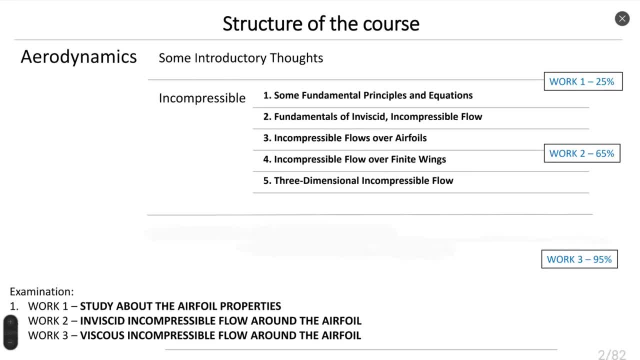 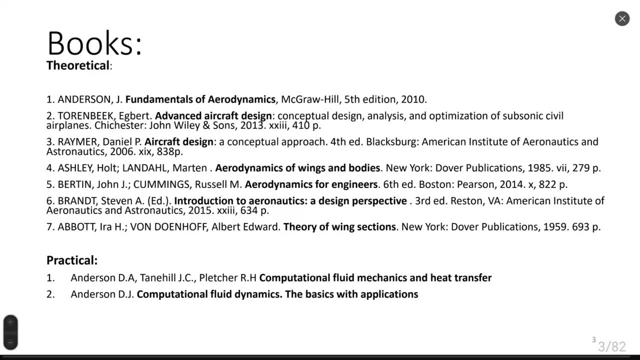 one week before end of the course. Here you can see a list of books which I recommend you 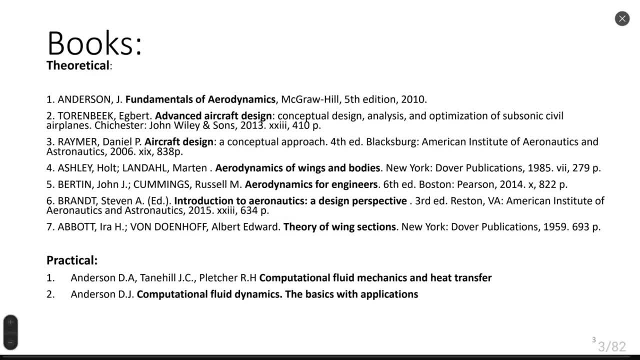 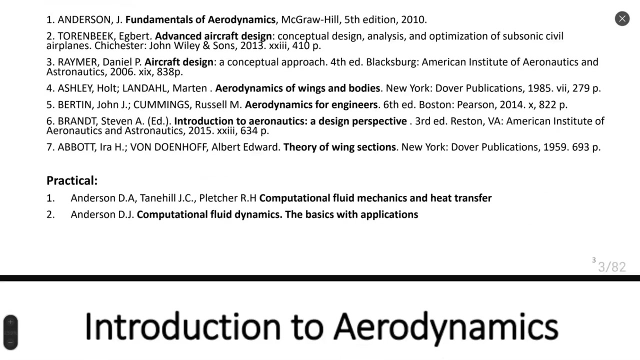 for studying of aerodynamics. The main book we will use is Fundamentals of Aerodynamics, of Anderson. You could use 5th or 6th edition of this book available in our library. And for practical classes I recommend you Anderson-Tonihill-Platcher as the base book, Computational Fluid Mechanics and Heat Transfer. And also you can find many other resources about aerodynamics in our library or in the internet. Aerodynamics is having already more than 100 years of use. 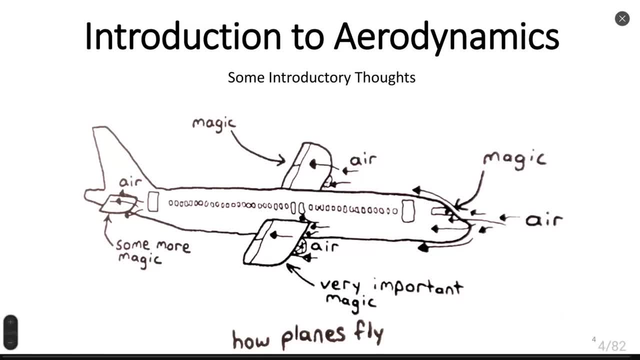 And it studies the magical forces which appear on airplanes and allow them to fly or allow them to resist to gravitational forces and take off. These magical forces we will study here in aerodynamics and our lectures will allow you to understand how to relate force and flow properties happening around the aerodynamic body. 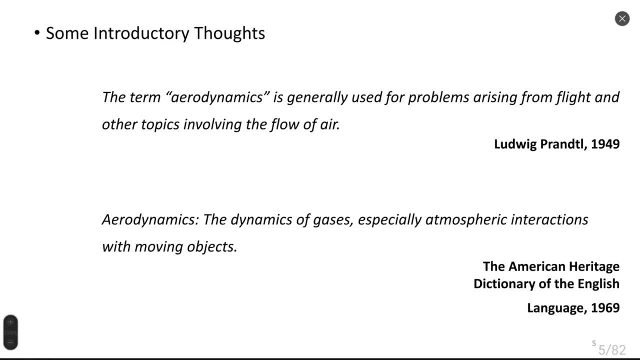 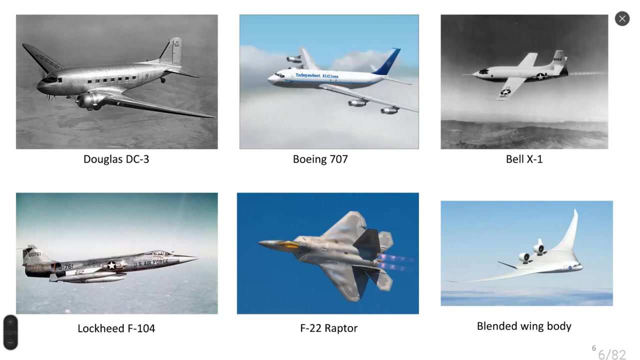 History of aerodynamics accounts for more than 100 years of development and many famous scientists contributed to it. Probably one of the most famous was Ludwig Prandtl and we will study in this course many of theories he has developed. Here on my screen you can see several airplanes which were developed with advancement of aerodynamics. For example you can see here Douglas DC-3. It's one of the most famous aircrafts of all times and it was a low-speed subsonic transport designed at 1930s. 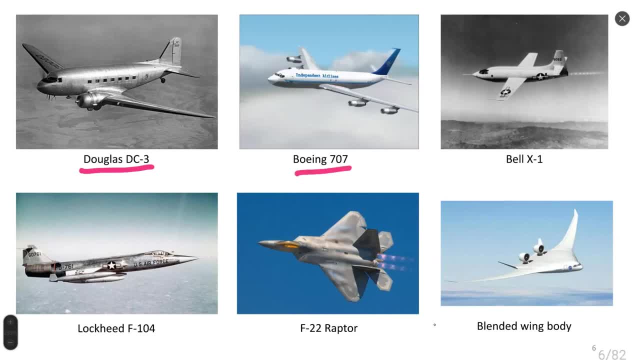 Then next one you can see Boeing 707. Which already flew at high speed the compressible regimes. And it allowed the transportation of millions of passengers in the late 1950s. 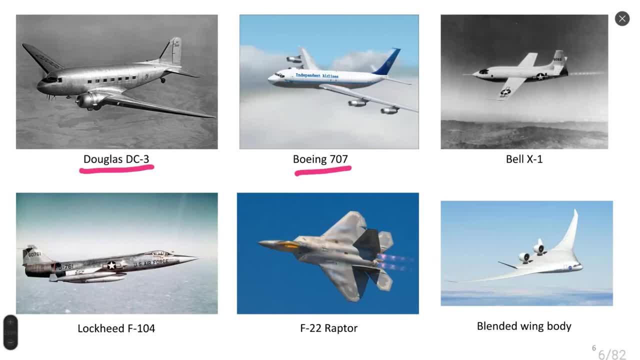 Then Bell X-1 was the first airplane flying faster than sound. 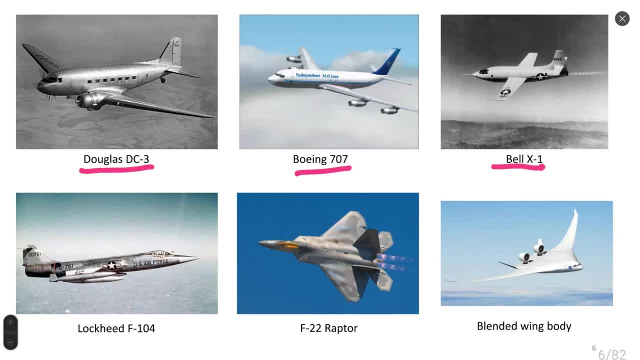 And Lockheed F-GC predictable- مinizу letzte ав duo таджикиijю faster than sound, and Lockheed F-104, which already flew with Mach 2, a huge advancement for time of 1950s. 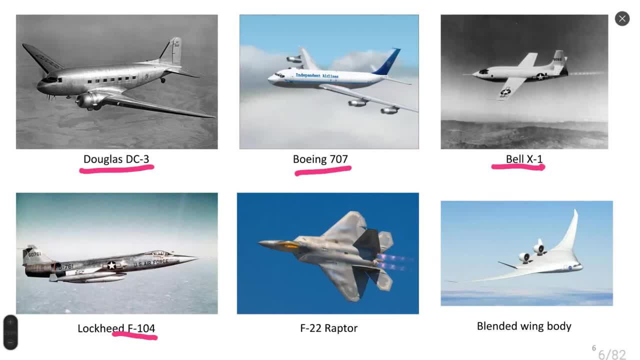 And with the development of computational method, it was possible to create airplanes which sustain long supersonic flights. 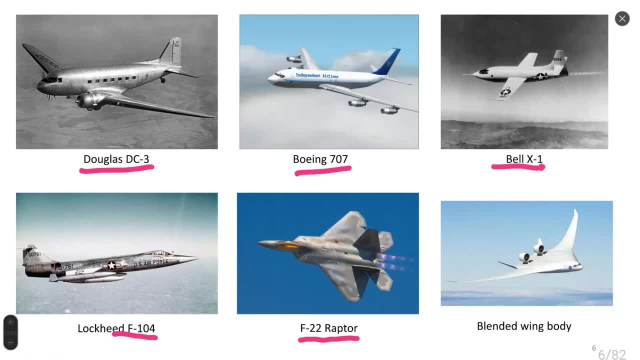 For example, Raptor F-22 is one of the most perfect airplanes for supersonic flight regimes. 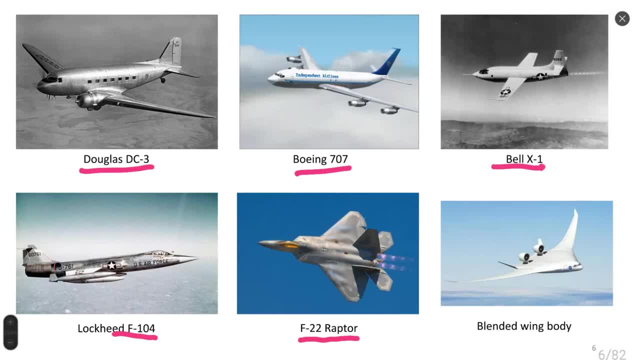 And finally, you can see a blended wing body, which is theoretically one of the most performant aerodynamics bodies which could be created, and this could be a future of aviation. 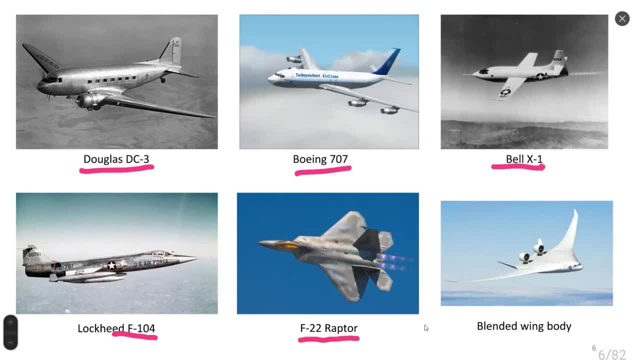 And, of course, advances in aerodynamics are not just limited by applications to airplanes. You know that flow of gases and flow of air is also very important in other fields. For example, civil engineering, flow around buildings, application to automotive engineering, flow around cars, flow inside cars, flow inside the engines. So, there are many applications. Thank you. 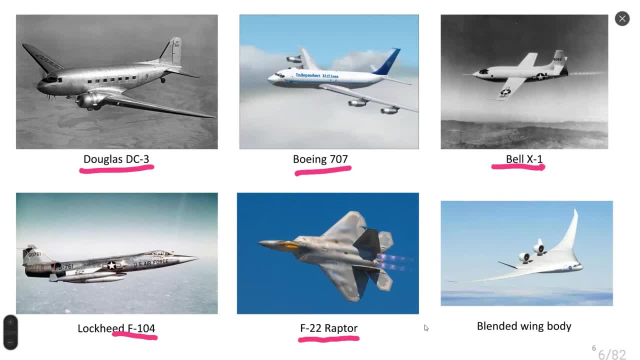 There are many applications where aerodynamics plays an essential role. 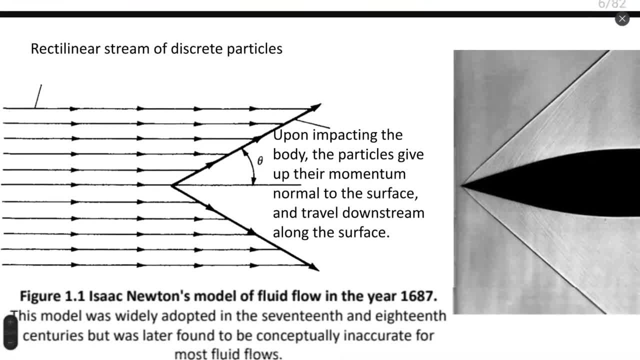 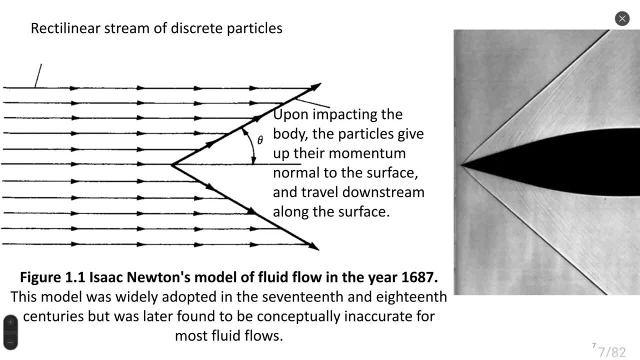 Now, I would like to talk a bit about historical examples in aerodynamics. One of the first work we can find in the literature is so-called Newton's theory, which was developed by Isaac Newton in 17th, 18th century, and it was trying to describe movement of fluid around an obstacle. This model... This model, as we might see on figure 1.1, is showing to us that fluid is moving undisturbed before it meets the body, and then suddenly it turns to an angle equal to the angle of the body. It was at that time an advanced theory, but after it was evident that theory is a completely different thing. 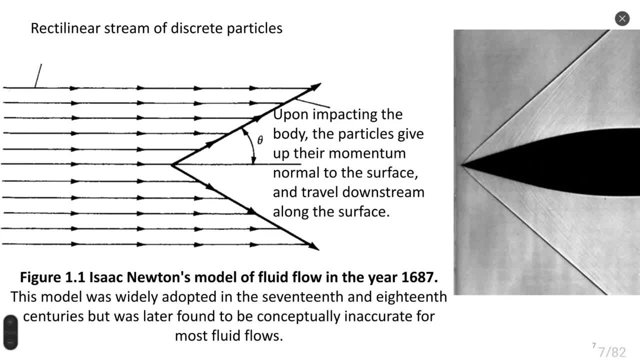 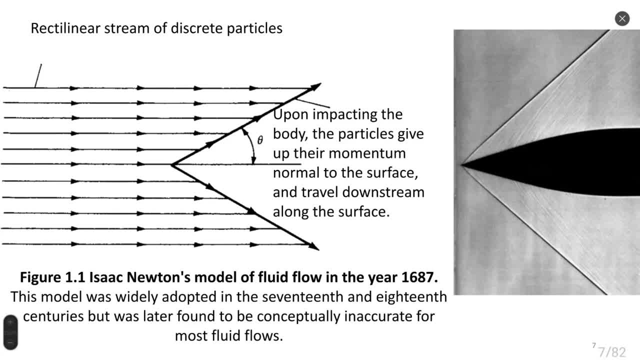 However, in 20th century, with development of supersonic and hypersonic flow applications, there were found some similarities with the theory of Newton and the movement of supersonic gases. 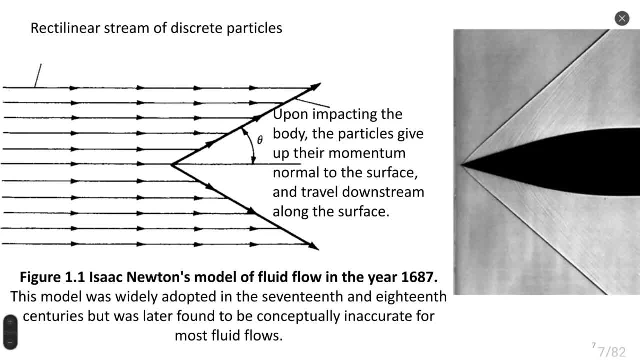 And this is one of the reason why one of the theories of hypersonic flow movement is called Newtonian theory. We will study it. study it at the end of gas dynamics in the chapter which talks about hypersonic flow applications 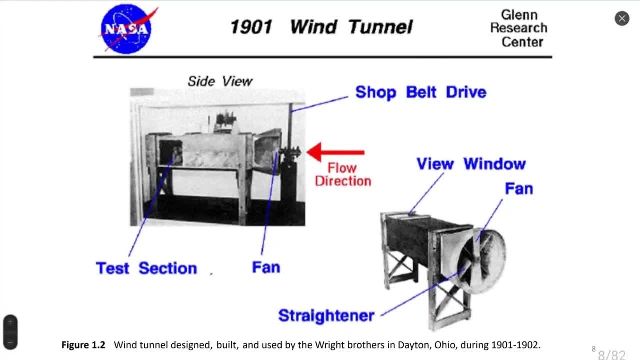 another very famous study of aerodynamics is provided by wright brothers in the united states which built a wind tunnel in order to find the best profile of the wing and build 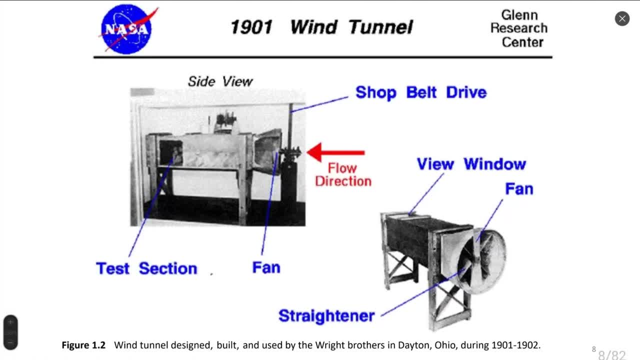 flying airplane this wind tunnel as you might see from this picture is consisting of test section where airfoils or wings were tested 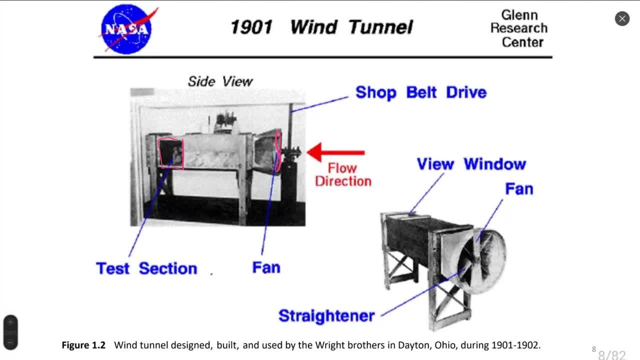 and a fan which accelerated the flow in axial direction 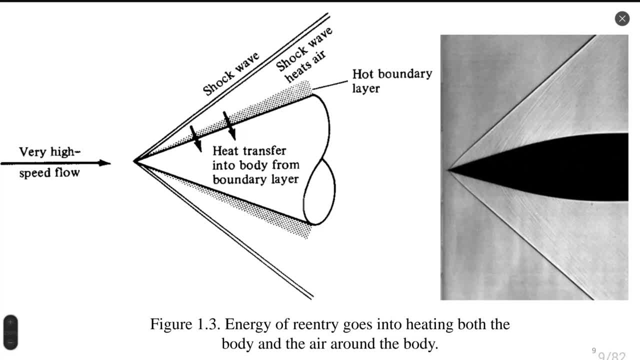 one of the very important advancement in aerodynamics and gas dynamics is development of theory of shock waves shock waves are present in flow that are moving with the supersonic velocity with respect to 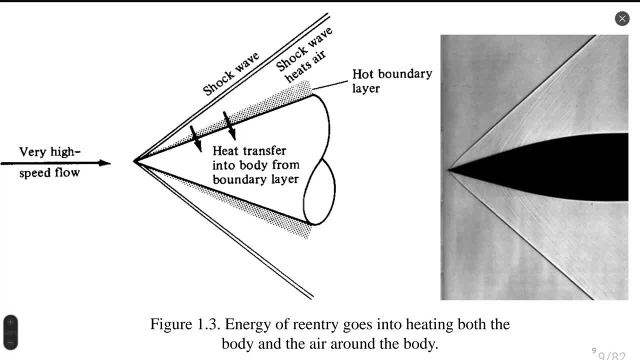 body and such interaction of flow and the body creates a rapid change of flow characteristics and flow patterns 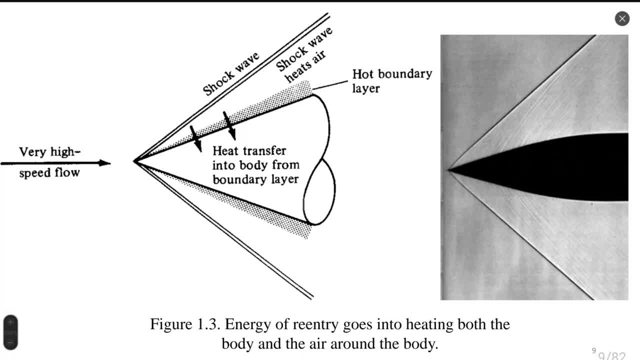 which we can consider as discontinuity and we call as shock wave shock waves can be of different type for example here on the screen you can see an oblique shock wave which is inclined with respect to the flow direction also in gas dynamics we will meet with another type of shock waves normal shock wave and the combination of oblique and normal shock wave 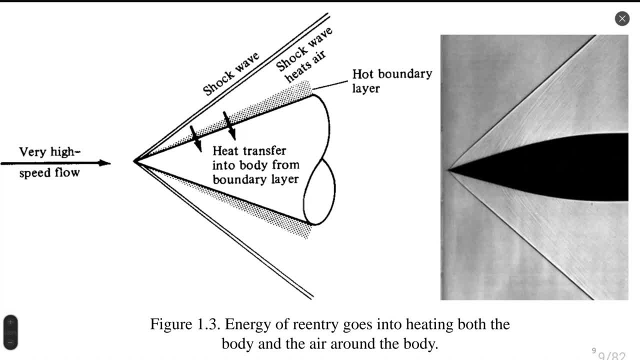 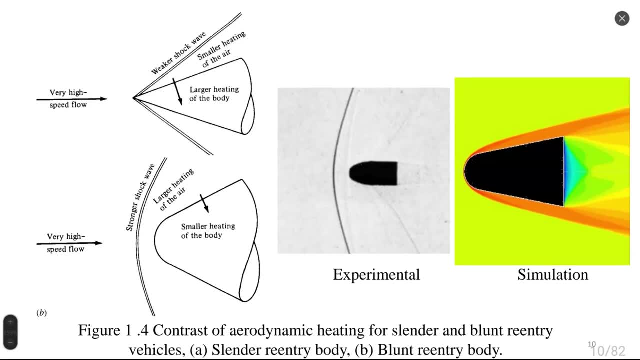 flow around supersonic blunt body is so-called bow shock wave bow shock wave you can see on my figure 1.4 flow around blunt re-entry body right uh actually this is one uh other advancement 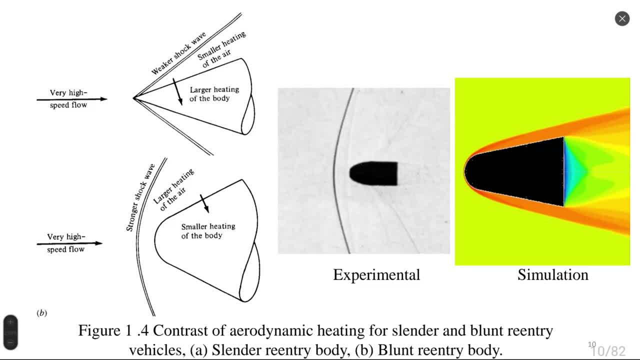 in aerodynamics that is an answer on a question which should be the shape of re-entry body not to burn in the atmosphere first of all uh we understand that a rocket or shape of the rocket or shape of the re-entry body could be of a different shape depending on this shape we can have different structure or flow around its body and we will have different properties of heat exchange of flow around the body and the surface by itself a big advancement in a theory of supersonic flow was made with the development 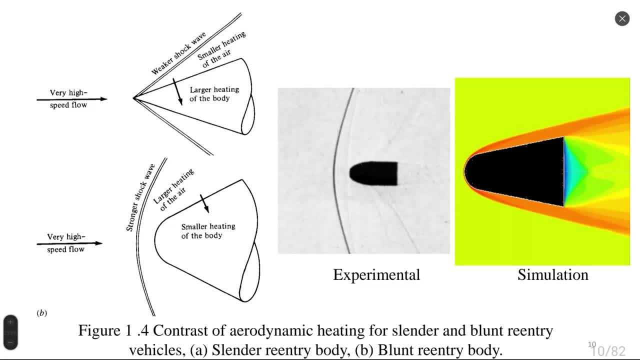 of plant re-entry body theory which is transforming or reconfiguring the balance between heat in the air for example here in figure 1.4 you can see on the upper part uh an oblique shock wave where there is a small heating of air after the shock wave but since we preserve the same amount of energy in the flow we will have larger heating of the body the total energy will be same in case of a blunt re-entry body we will have a different shape of shock wave as a consequence we will have larger heating of the air and we will have slow slower velocity of this air and as a consequence of this low velocity and large heating of the air we will have smaller heating of the body with respect to an oblique shock wave such flow structure can be absorbed experimentally you can see it in the middle of my screen and such flow structure can be absorbed also numerically by numerical simulation 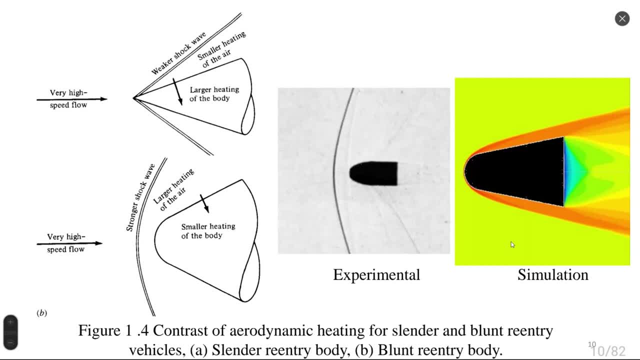 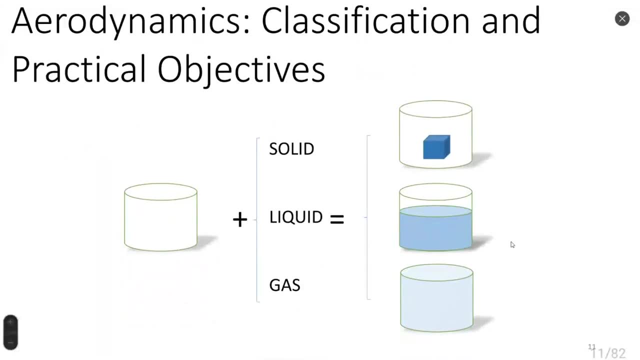 of ricochet methods ис타р villa sone or computational fluid dynamics which we also will study in the future 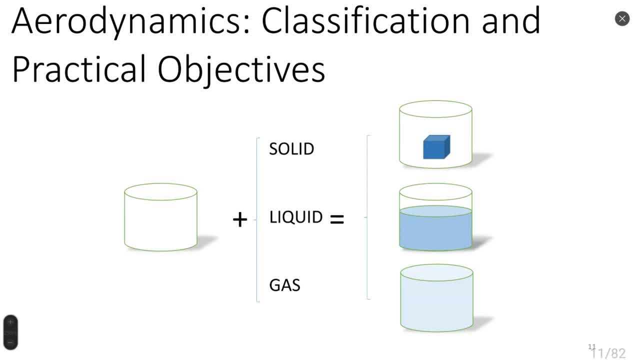 next we must talk about classification and practical objectives of aerodynamics we see that when solid is interacting with the liquid is fluid dynamics interacting with air is called aerodynamics and the interaction of solid body with gas 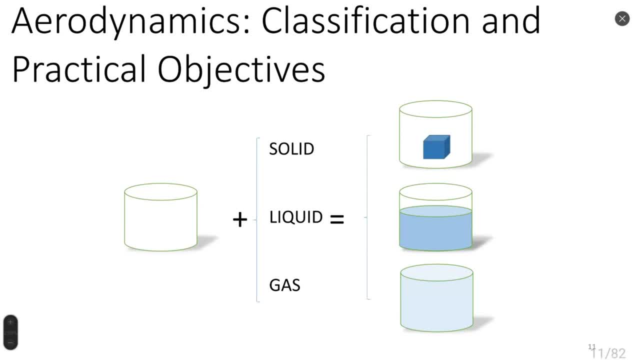 in general is called gas dynamics also inside gas dynamics we include compressibility effects so compressible aerodynamics is usually also called gas dynamics 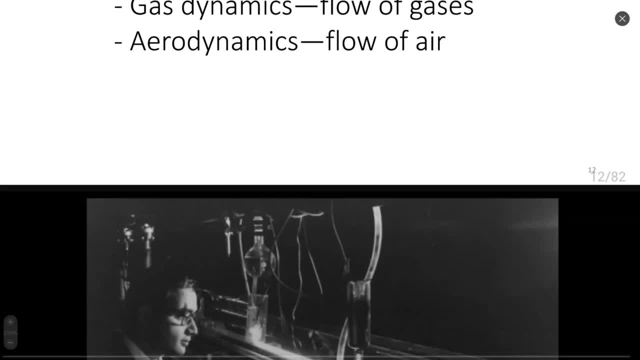 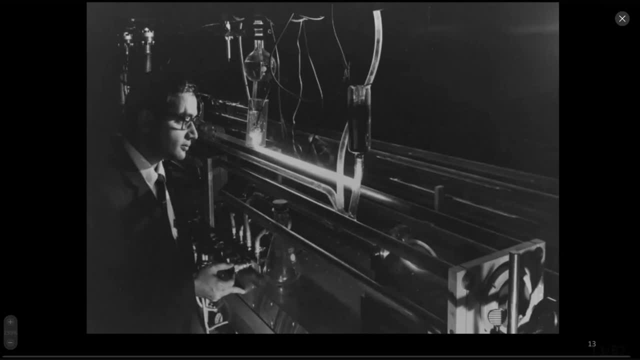 here is written what i just said you on the previous slide and here is the scientist working on gas dynamic laser one of motivating picture 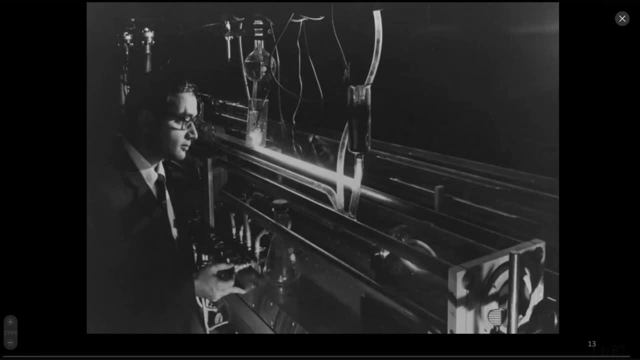 which should help you to understand importance of aerodynamics theoretically 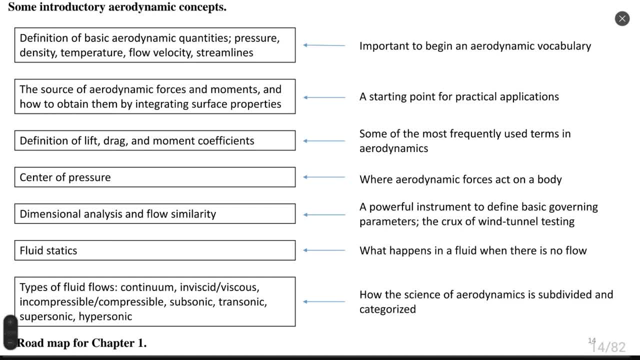 okay here is the road roadmap for chapter one of aerodynamics here we see definition of basic aerodynamic quantities like pressure density temperature flow velocity streamlines we see how to quantify how to find equation of these quantities then we see the source of aerodynamic forces and moments and how to obtain them by integrating surface properties like pressure and shear stress then we will define the general reaction force and its division on lift drag axial normal components and momentum coefficient 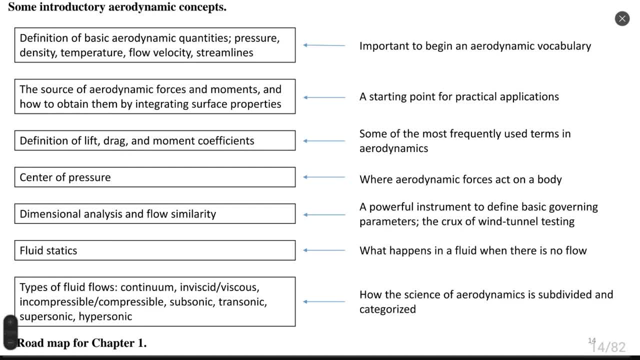 then we will see how to calculate center of pressure on aerodynamic body after doing this we will find a way how to make dimensional analysis which would help us to find relation between for example test of a model of the airplane in aerodynamic tunnel and real flight 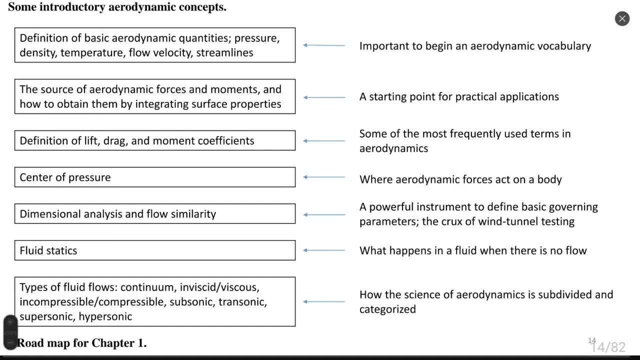 conditions then we will talk about fluid statistics what is the flow rate of the airplane 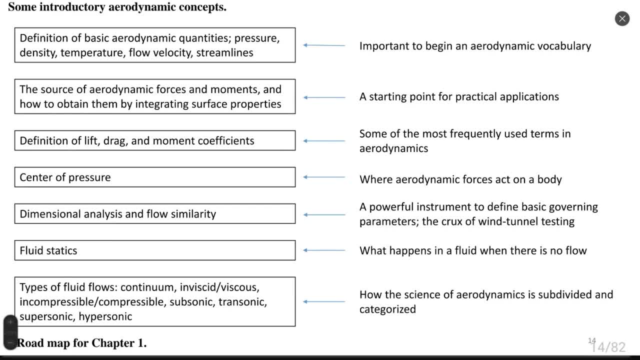 happens when there is no flow it's quite short topic and at the end we talk about types of fluid flows continuum flows inviscid viscous flows and compressible compressible flows subsonic transonic supersonic and hypersonic regimes it's a kind of reminder for you for people who had 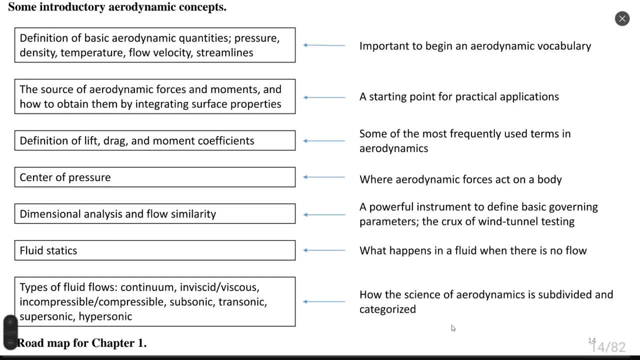 work with the fluid mechanics for example or fluid dynamics some time ago for people who just finished fluid mechanics and fluid dynamics this would be very very simple topics okay the first part of chapter one is fundamental 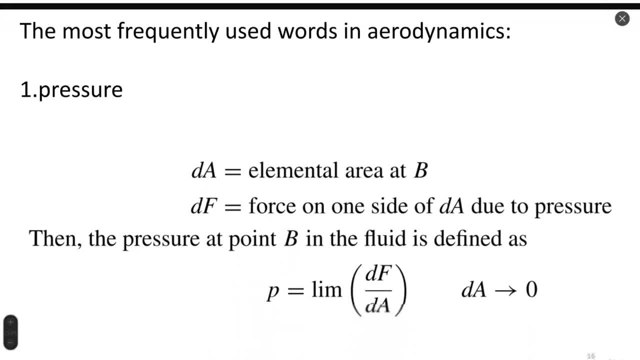 aerodynamic variables these fundamental aerodynamic variables are scalar or vector values 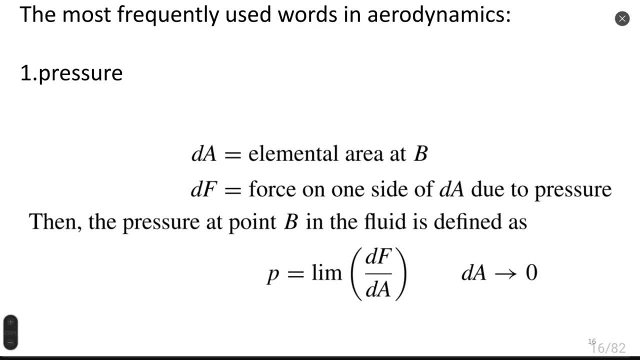 maybe one of the most important is pressure is defined as the limit of ratio of 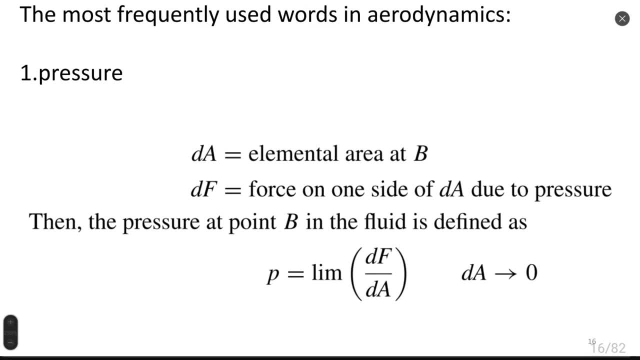 force elementary force on the elementary area relation pressure can be seen inside the fluid or on the body surface 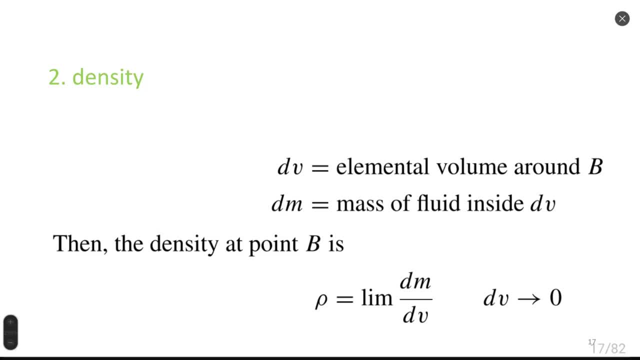 then we have definition of density which is limit of mass differential by the volume differential density has dimension of kilogram per meter cubic 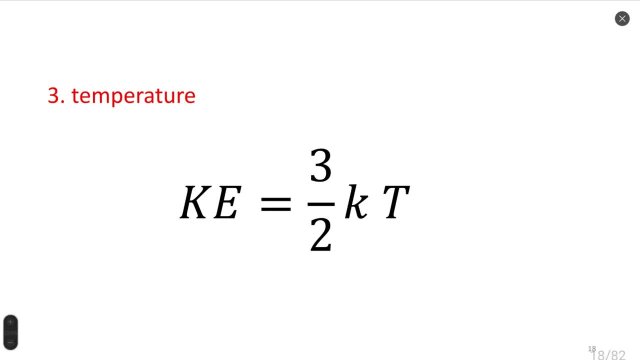 and temperature which can be defined by the kinetic energy of gas through the boltzmann coefficient and also temperature can be defined by the equation of state of gas if you know there is a 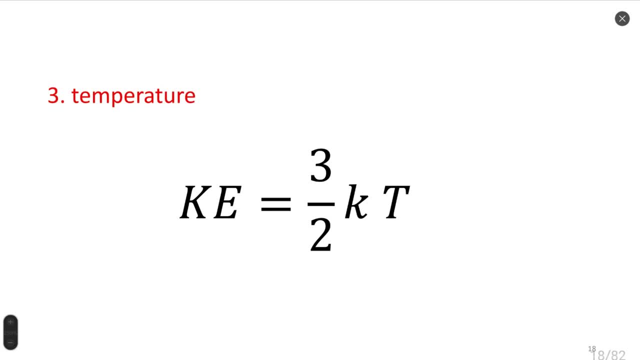 relation written as pressure equal to density multiplied by gas constant multiplied by 10 temperature where temperature could be calculated from this equation to use this equation do not forget that we must have all quantities in c units for example pressure in pascal density in kilogram per meter cubic gas constant in joule per kelvin per kilo 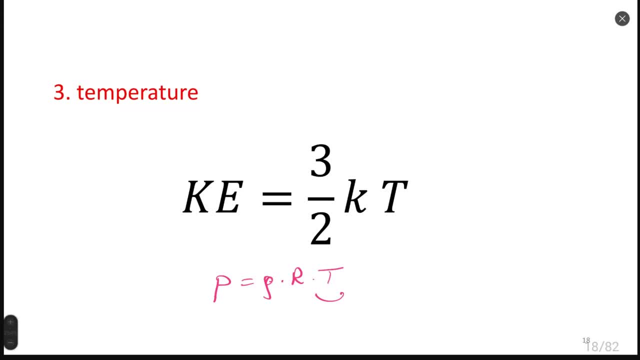 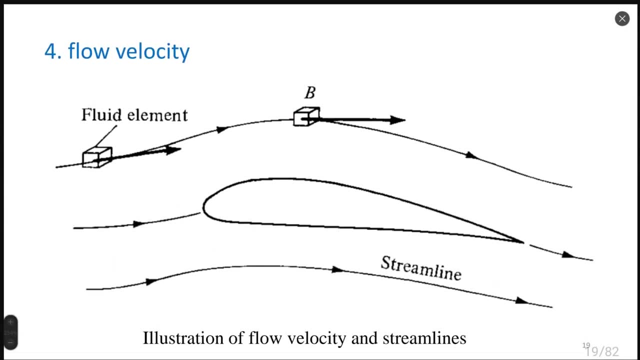 gram and temperature would be calculated in kelvin as a vector property we have a flow velocity which shows us direction of movement of fluid at any point probably if you remember fluid mechanics you know that this fluid velocity could be different for any any point in space as well as any scalar property like pressure temperature and density okay all right i'm going now to give you's a little freely Weather 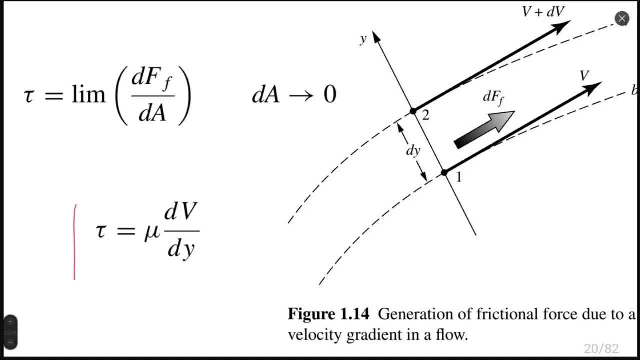 شير stress happier course then let's see since it is a less elements Schroedcher equation He told his student here that shear stress would be proportional to dynamic viscosity coefficient multiplied by gradient of velocity in the direction normal to the electric field minus glue and here we Learning that the gradient of ferminity of the field increase andобразed 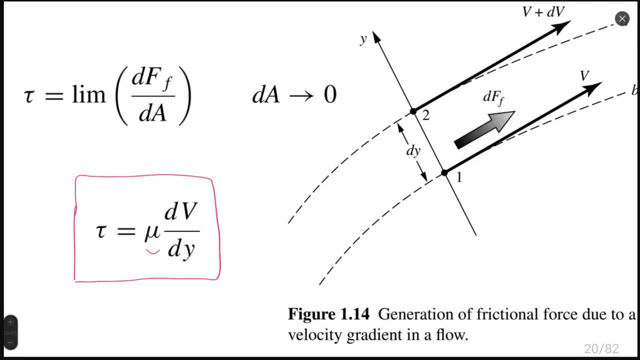 in direction normal to Share stress to the wall where y direction is it is direction of perpendicular to the wall of body usually shear stress we have inside boundary layer where velocity gradient has considerably high value outside of boundary layer where velocity is approximately same everywhere 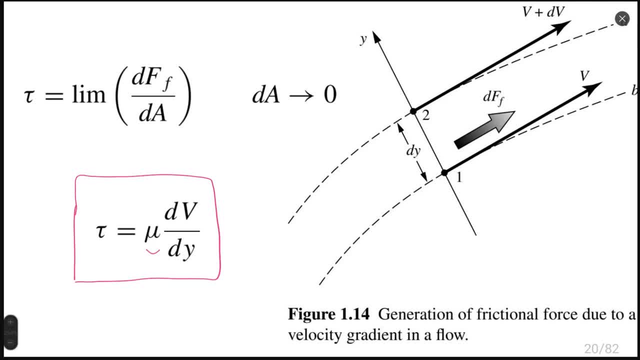 shear stress would be negligibly small with respect to pressure forces 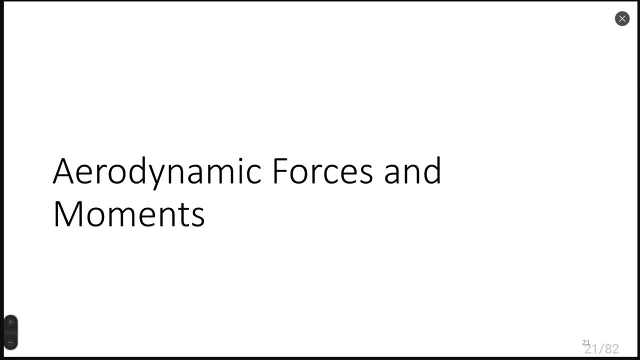 okay once we talk about thermodynamic and aerodynamic properties we can speak about aerodynamic forces and moments what are these forces and moments 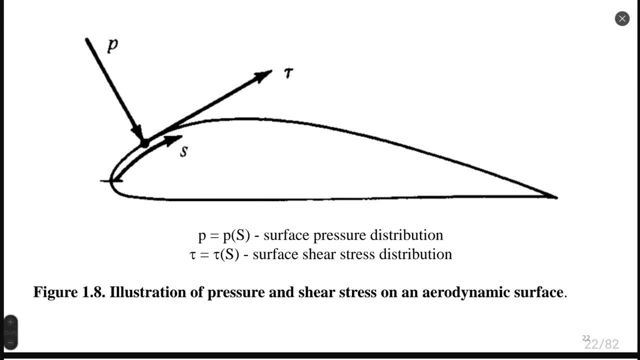 the source of aerodynamic forces and dynamic moments pressure and shear stress distributed on the surface of the body. 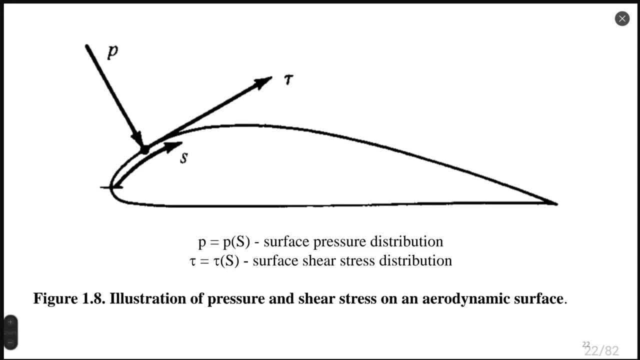 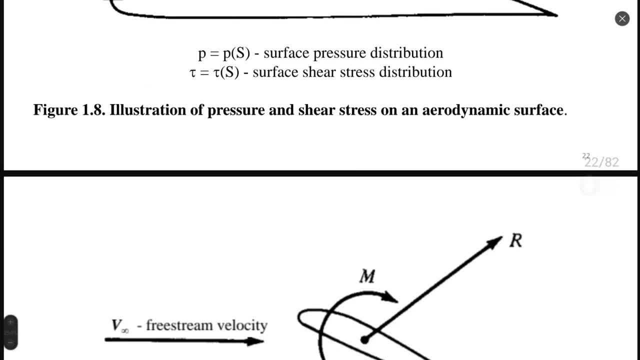 We know that pressure force is always perpendicular to the body surface and shear stress is tangential to the surface. Once we integrate, which we will see very soon, 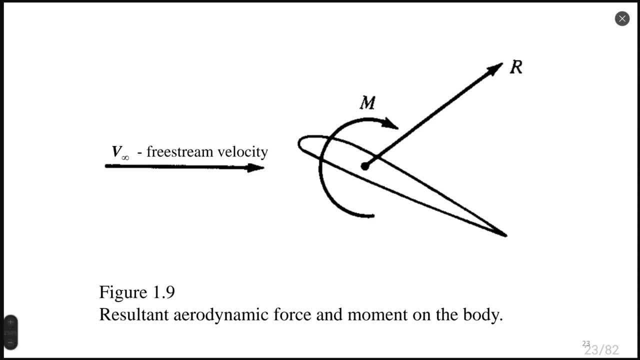 these forces will result in momentum and reaction. 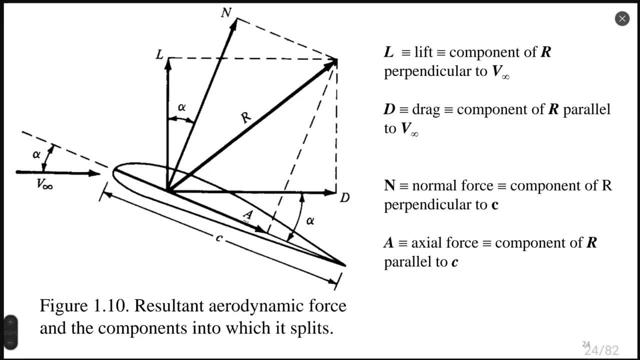 After we obtain reaction force, we can split it in various combinations of forces, which would be probably perpendicular forces. Here you can see on this screen there is a reaction force as you can see. 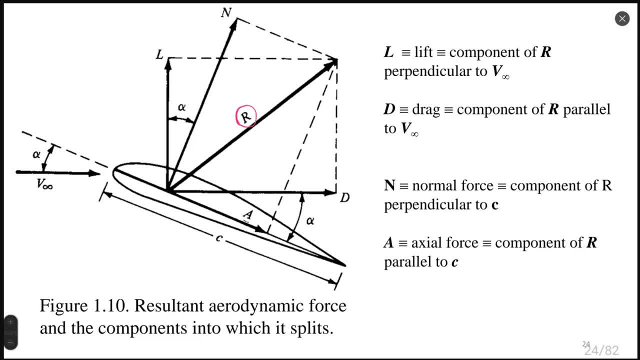 A total of all influence of pressure and shear stress on my airfoil and this reaction force 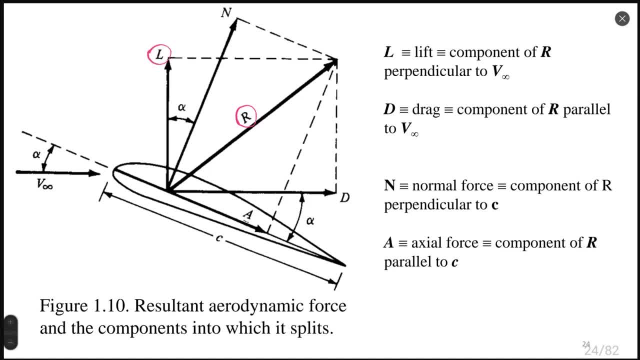 could be split to lift, for example, and drag. Lift is L and drag is denoted as D force. Lift and drag forces are perpendicular one to another. Lift force is a force which is also perpendicular to the infinite velocity. 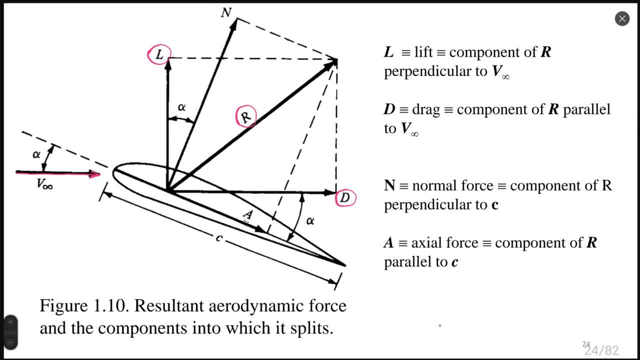 Here you can see it on figure 10. So lift perpendicular to V infinite 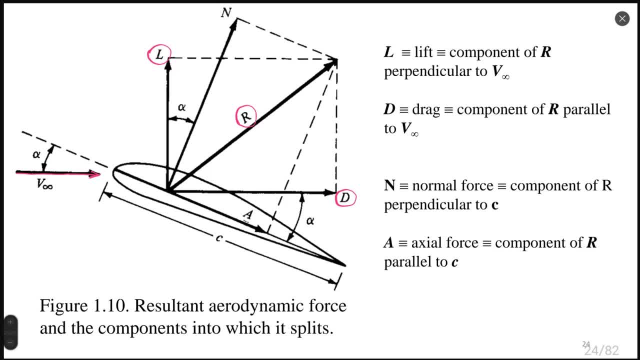 and since lift and drag are one perpendicular to another, drag is parallel to velocity vector. 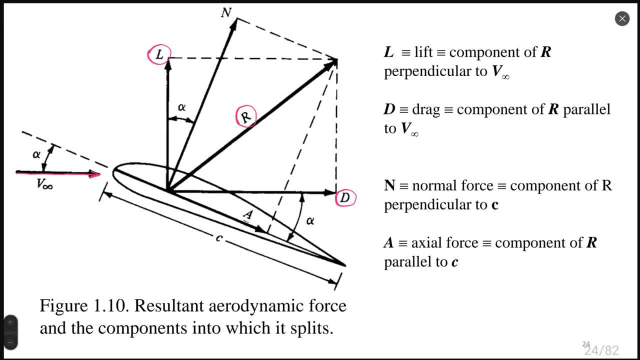 Then when we will work with the aerodynamic quantities, sometimes it's useful to split reaction force to another pair of vectors which are called normal force and axial force. Axial force is the force which is going parallel to the main horde of airfoil. The horde is the line straight line which joins the starting point of airfoil called leading edge and the final port point of airfoil called the trailing edge. So the starting point of the airfoil is the leading edge and the trailing edge. And parallel to axial force we have a normal force. Perpendicular to axial force we have a normal force and it's also perpendicular to a horde. Transition between normal axial force and lift and drop force can be easily seen by trigonometric relations once we introduce angle between these pair of forces. As you can see this angle is denoted as alpha. You can see this angle also between infinite velocity and direction of airfoil is alpha on the left. This alpha also can be seen between lift force and normal force. 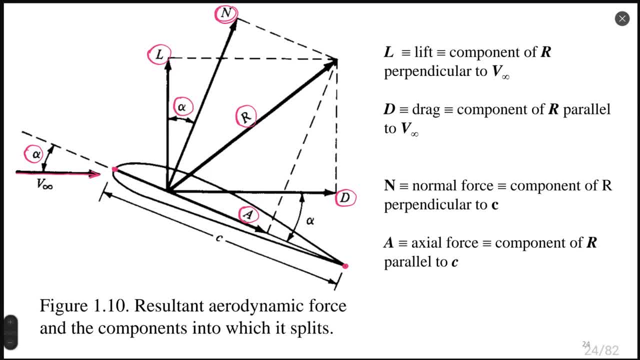 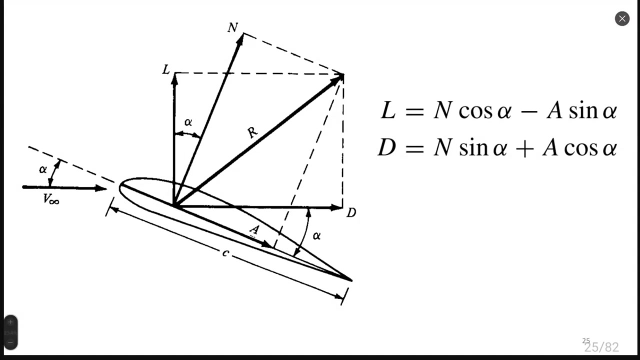 And because all these angles or forces are creating similar triangles, this alpha can be observed between axial force and drag force. As I already told you the resultant force is R. So writing in vector form we can have the following relation that R is L plus D and it's same as n plus a vectors. Based on this vector relation we can find the relation between lift, drag, axial, and normal force. For example, this relation between lift, how to calculate lift and drag when we know normal and axial forces are shown on this slide here. We can see that lift force must be or can be calculated by taking normal force value multiplied by cosine of alpha minus axial force multiplied by sine of alpha. And the drag force can be calculated as normal force multiplied by sine of alpha plus axial force multiplied by cosine of alpha. This can be also seen or visualized based on our schematic of forces which you can see here. For example, let's see that lift force, how much would be when we take a normal force multiplying it by cosine of 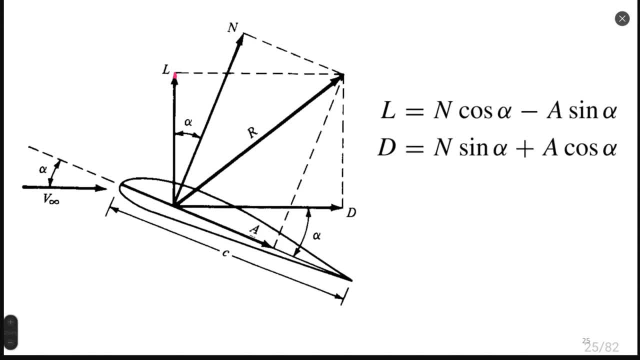 alpha. Let's see what it gives to us. I will make a projection on lift force direction. So my n multiplied by cosine of alpha would be this big vector starting at the origin of coordinates and finishing at the top. So it's more bigger, it's bigger than my lift force, this first part. 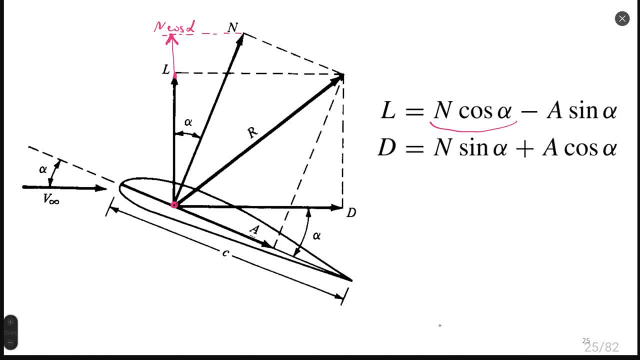 And cosine of alpha. So I need to subtract some value, this value which you can see on my screen, and this would be exactly axial force multiplied by sine of alpha. So let's make projection again to the direction of lift force. And here it is. Since my axial force is going down, it will generate projection vector also going down. And this projection vector would be equal to a multiplied by sine of alpha and it will be exactly the vector which i needed to subtract from my first vector n cosine alpha as the result i receive a lift force 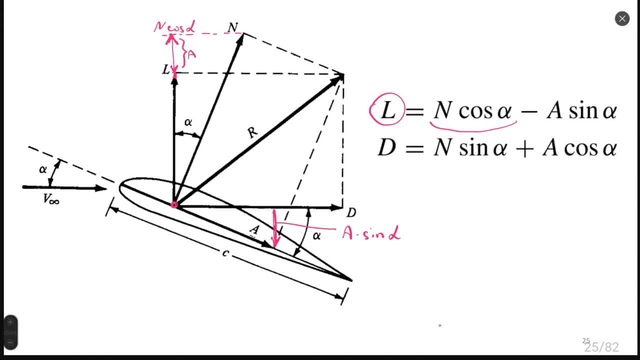 so this is a sine of alpha and for the drag force we can do the same we just need to project a normal indexial force on direction of the drag force so let's do this example here let's project normal force this is i will try to do it 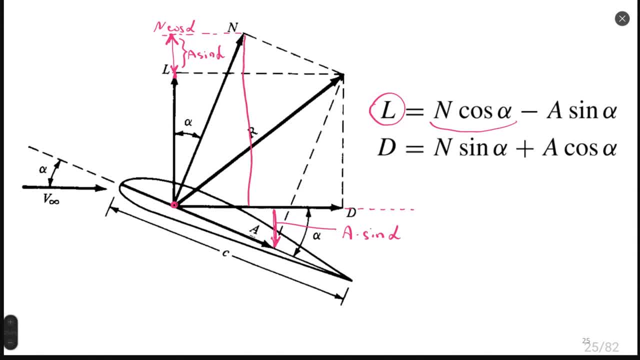 carefully okay this is the projection line and this is the force so i will denote it as 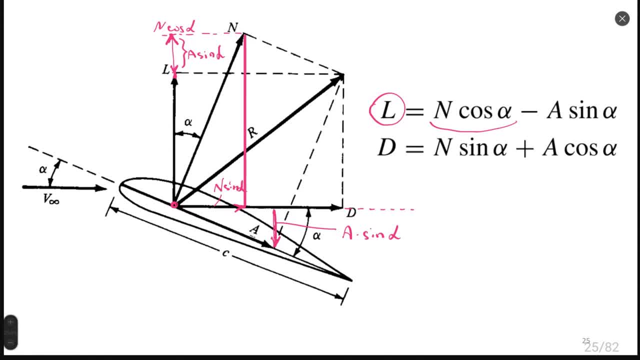 n sine of alpha so there is missing a big part and this big part i will obtain projecting axial force on drag and i will receive this big 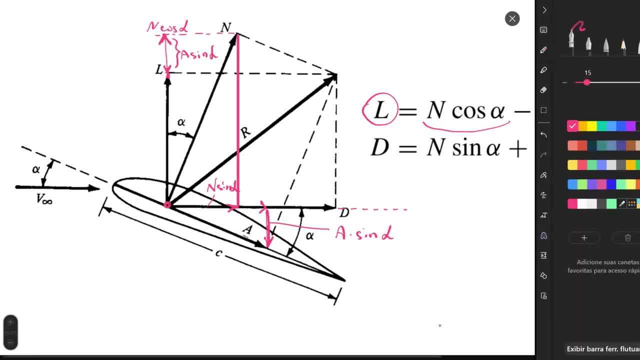 vector here i will make it by another color just for better visualization 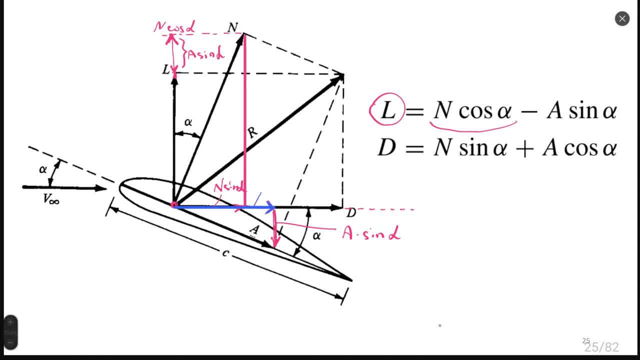 so this is my a cosine of alpha when i sumate this n sine alpha and a cosine alpha i will receive my drag force this is how transformation can be done and such transformation can be provided also in reverse direction from 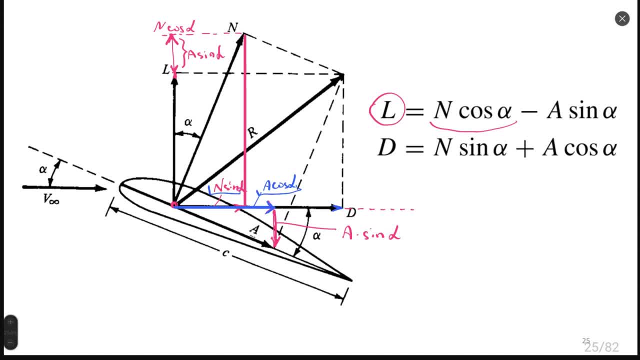 lift and drag forces we can obtain normal and axial force